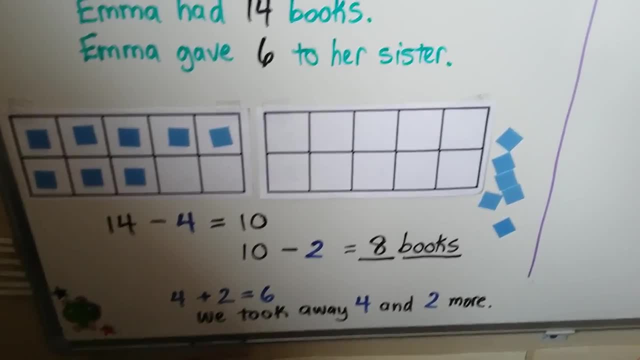 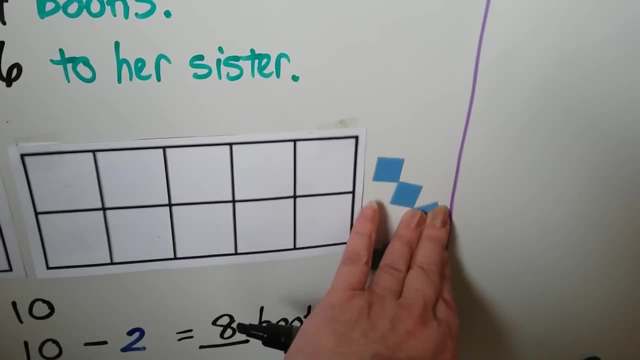 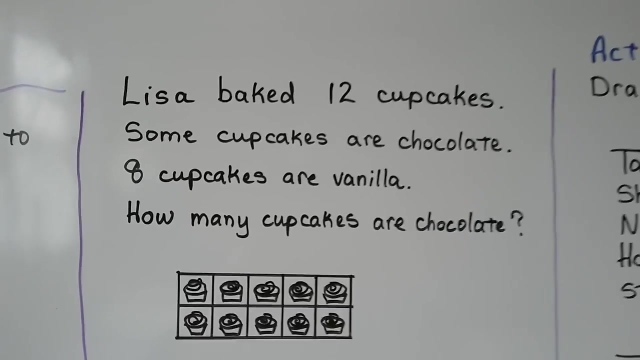 the four minus one plus two equals six. So we took away four and two more. We took away one, two, three, four, five, six. We took away these six. Lisa baked 12 cupcakes. Some cupcakes are chocolate, eight cupcakes are vanilla. 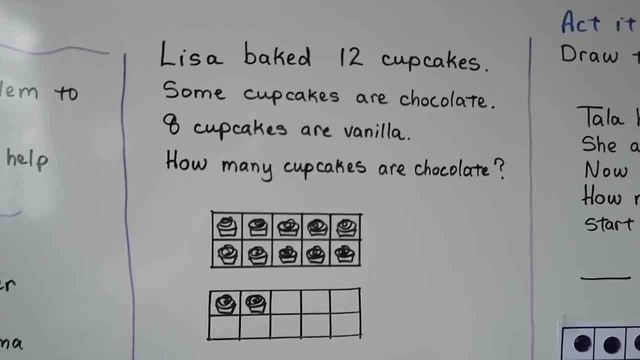 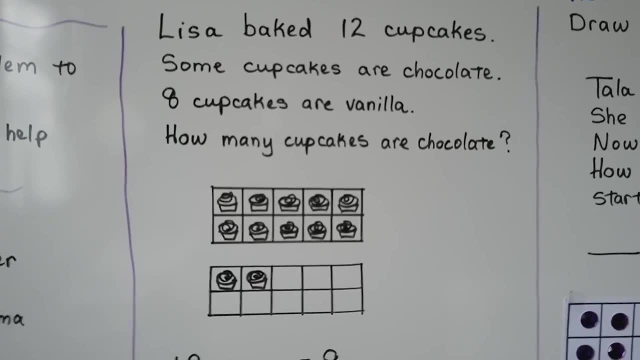 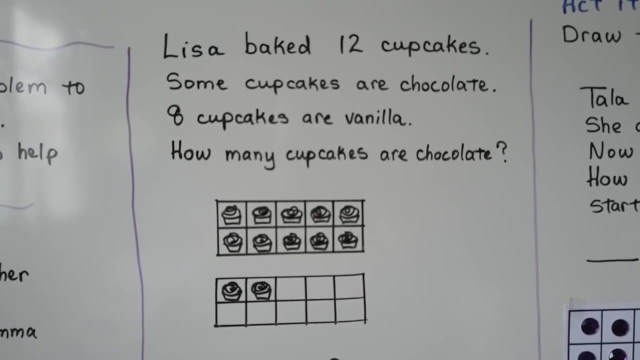 So how many cupcakes are chocolate? So what do we need to find? Well, we need to find how many or chocolate. The question, And what information do we need to use? We need to use that there were 12 and 8 are vanilla. And how will we use the information? Well, we can use a 10 frame and 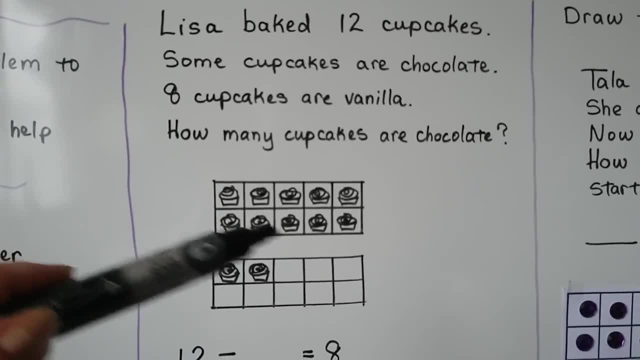 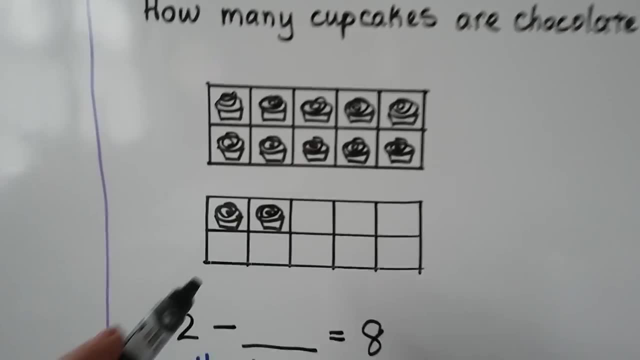 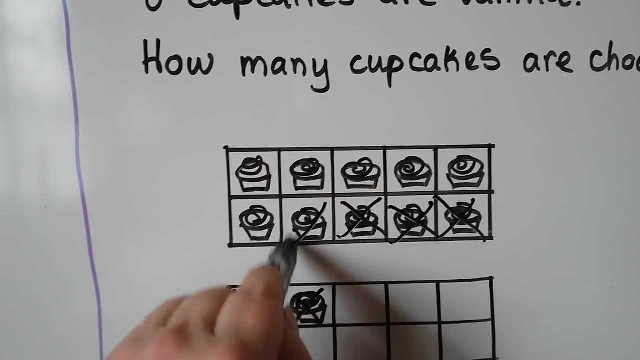 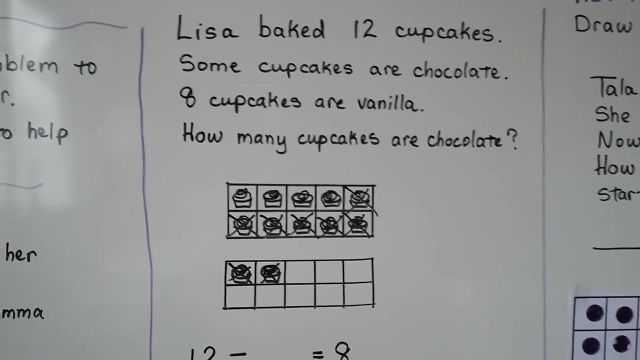 help us act it out. There's 12 cupcakes: 10,, 11, 12.. 8 are vanilla, So let's cross out the vanilla ones: 1, 2, 3, 4, 5,, 6,, 7, 8.. So we crossed out the vanilla ones. That means the rest are. 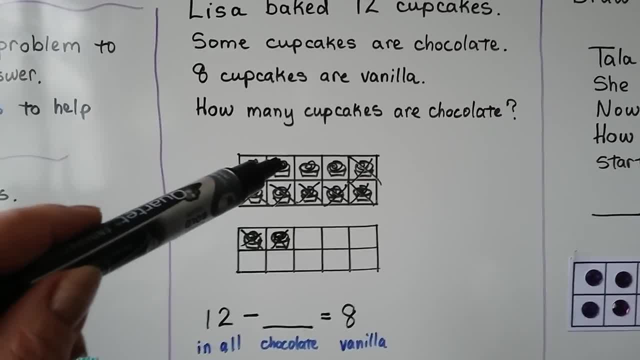 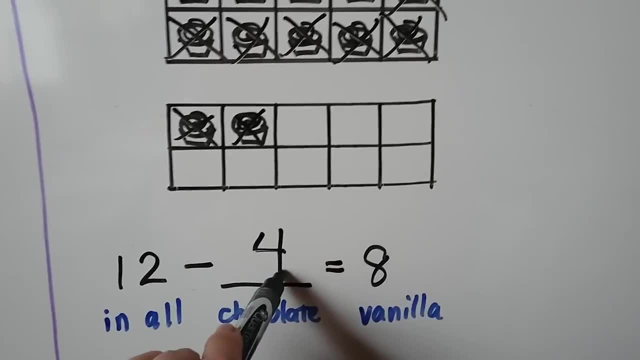 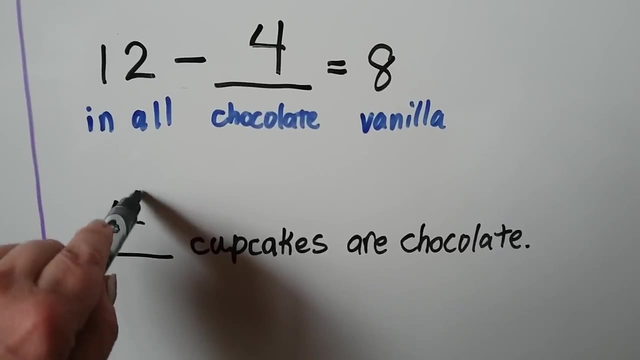 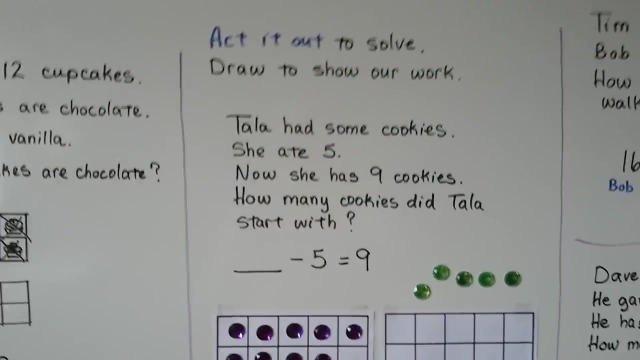 chocolate. How many are chocolate? 1,, 2,, 3, 4.. There's 12 in all. 4 are chocolate And that equals 8 vanilla, 4.. 4 cupcakes are chocolate. 12 minus 4 is equal to 8.. We can act it out to solve and draw to show. 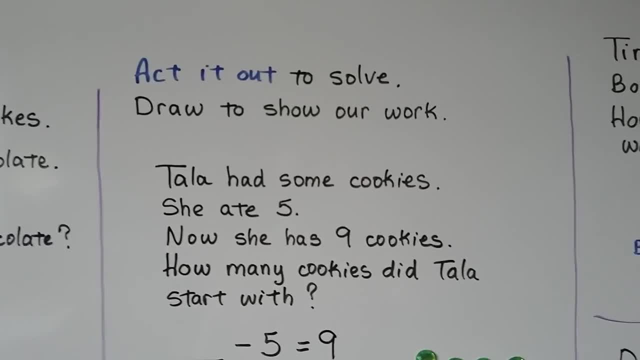 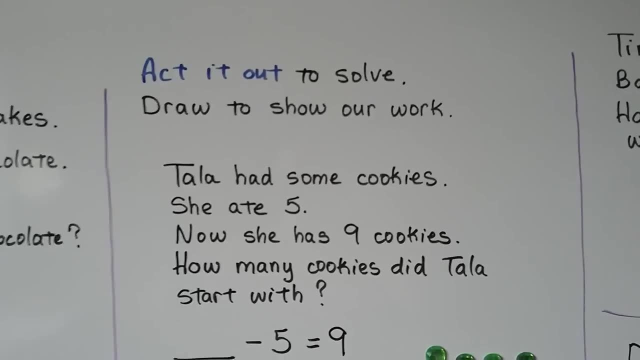 our work. Tala had some cookies. She ate 5.. Now she has 9 cookies. How many cookies did Tala start with? Well, it doesn't tell us. It just says that she has some cookies. So what do we? 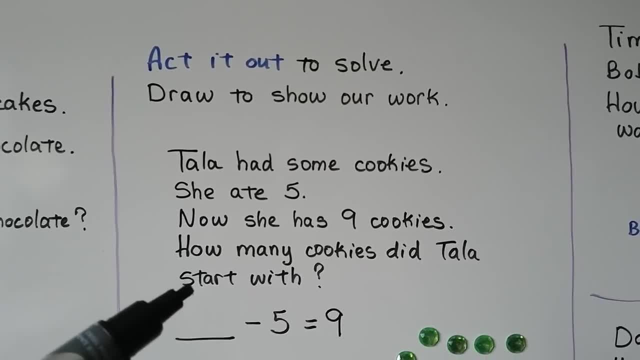 need to find. We need to find how many cookies she started with. We need to find how many cookies she started with. We need to find how many cookies she started with. What information do we need to use that she ate 5 of the bunch of? 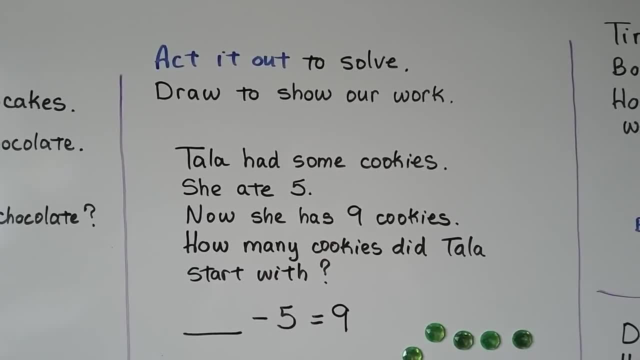 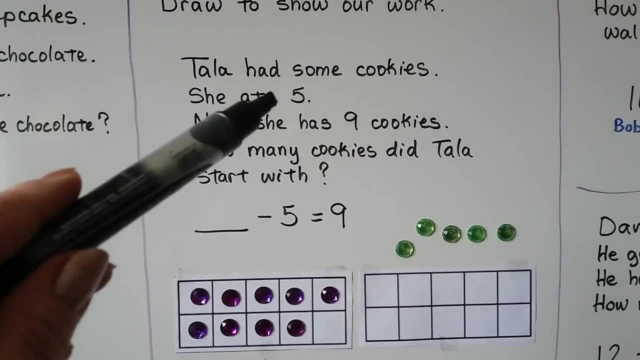 cookies and now has 9 left over. And how will we use this information? Well, we can make 10 frames to help us act it out. We we know that she ate 5 and she has 9 left over. So here's the 9. 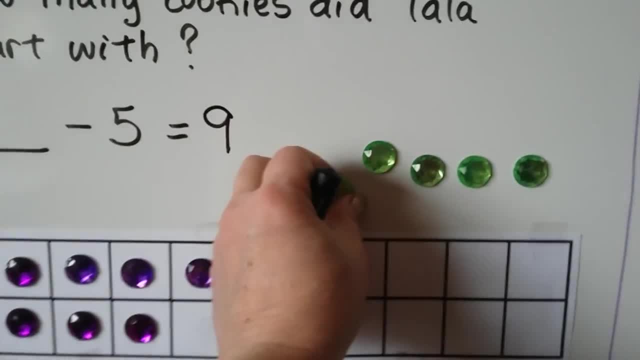 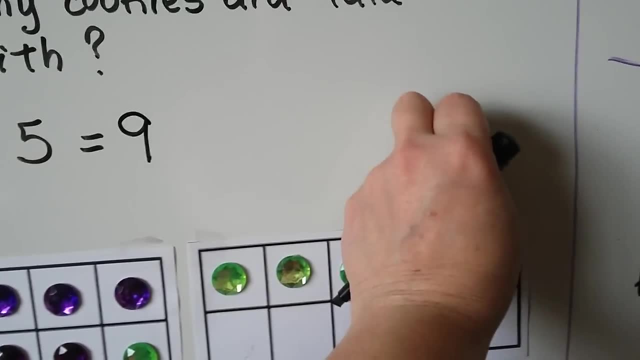 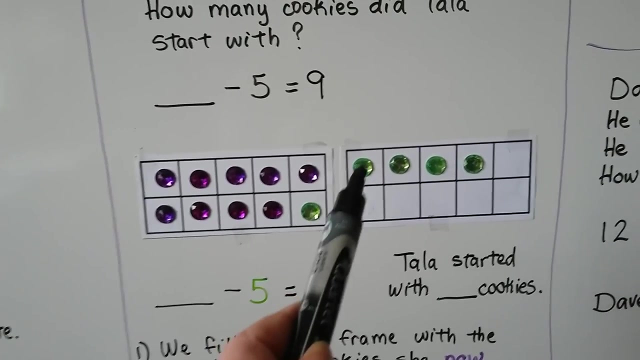 that she's got left over. We can put the 5 that she ate- 1, 2, 1, 2,, 3,, 4,, 5, and we can figure out how many. she started with: 10,, 11,, 12,, 13,, 14.. 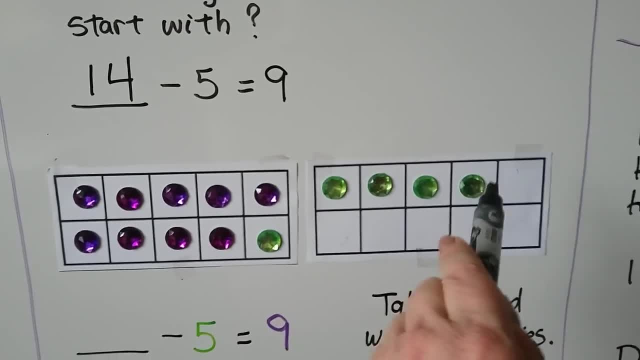 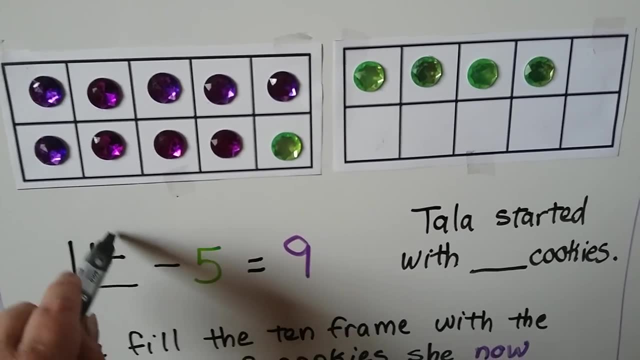 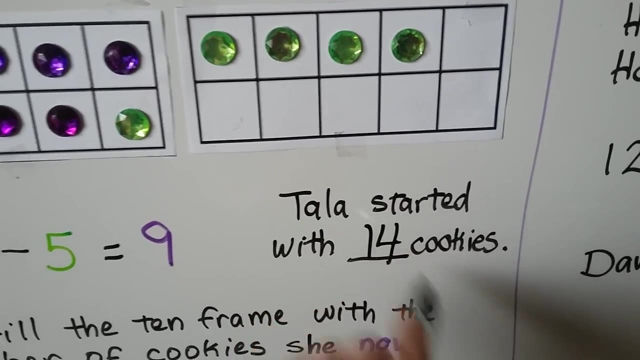 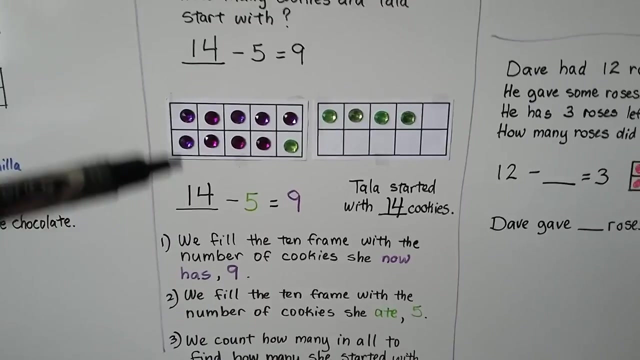 If we have 14 and we take these 5 away, we will have 9 left. 14 minus 5 is equal to 9.. So Tala started with 14 cookies. We fill the 10 frame with the number of cookies she now has. 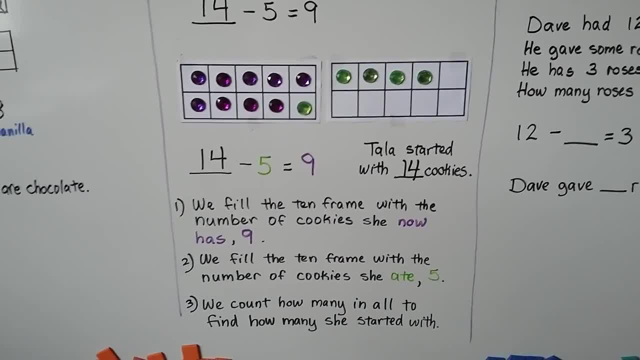 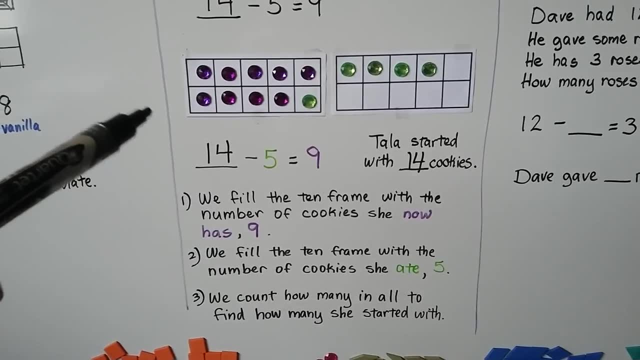 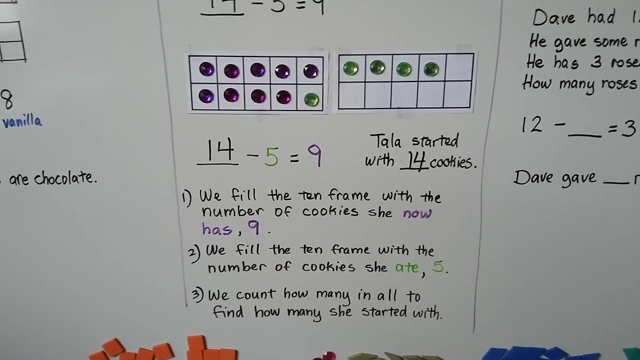 It says she has 9 cookies. So we put 9 purple markers or any color. We fill the 10 frame with the number of cookies she ate. She ate 5. And we count how many in all, to find How many she started with. 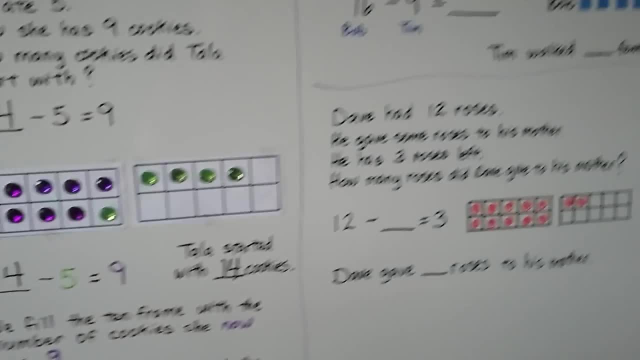 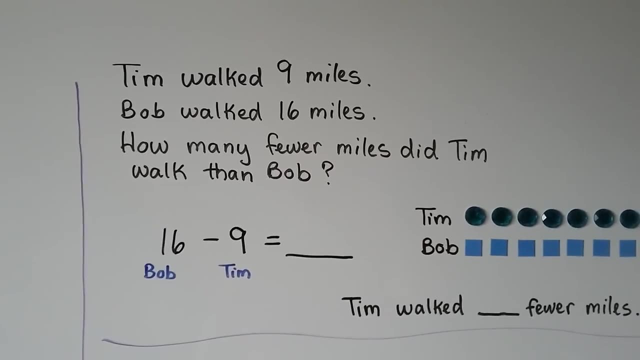 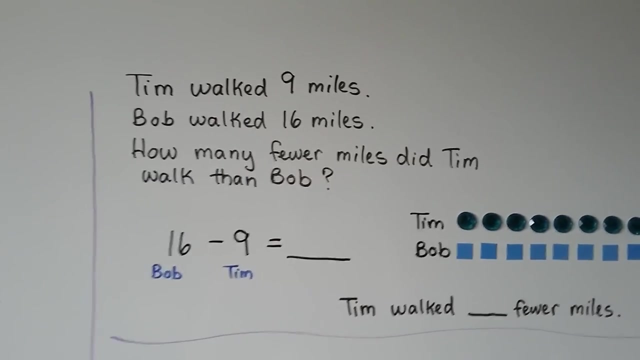 She started with 14.. Tim walked 9 miles. Bob walked 16 miles. How many fewer miles did Tim walk than Bob? The word fewer tells us it's going to be a subtraction sentence, A subtraction problem. So what do we need to find? 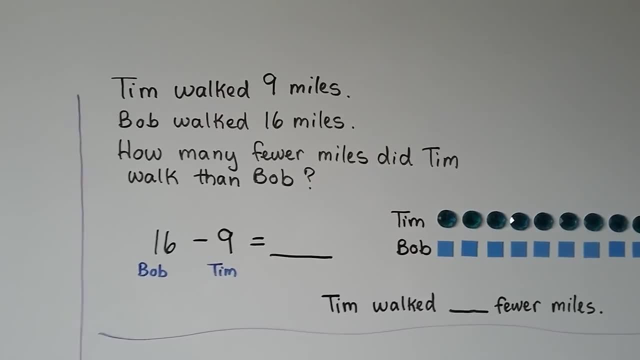 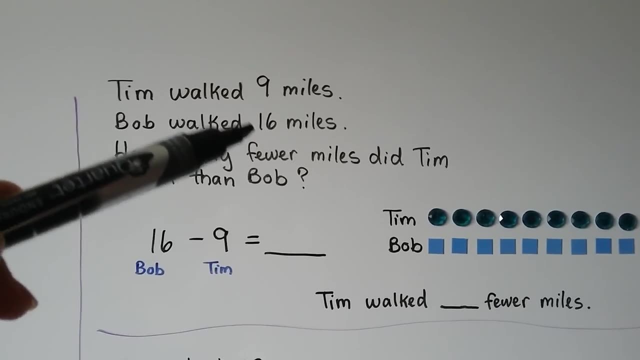 We need to find how many fewer miles Tim walked than Bob. We can see Bob has a bigger number. So what information are we going to use? We're going to use: Bob walked 16 and Tim walked 9.. And how will we use it? 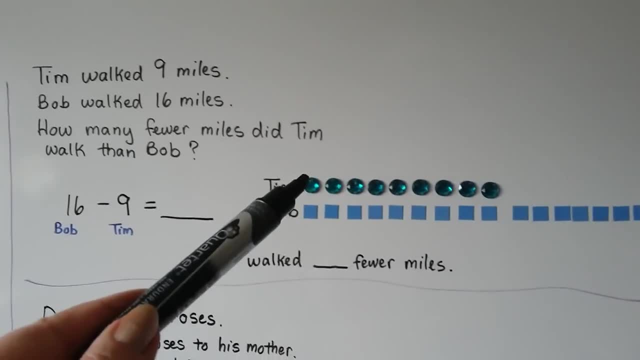 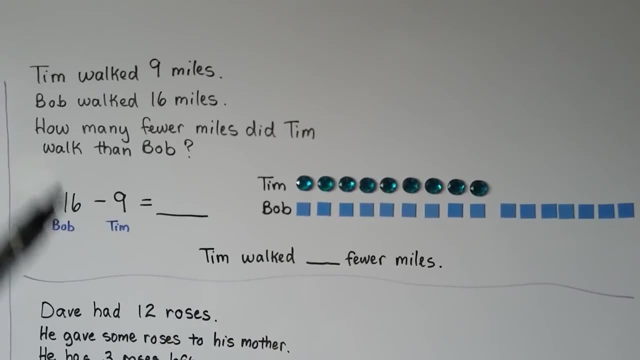 We can act it out with counters. We can give Tim 9 counters: 1,, 2,, 3,, 4,, 5,, 6,, 7,, 8,, 9.. We can give Bob 16 counters. 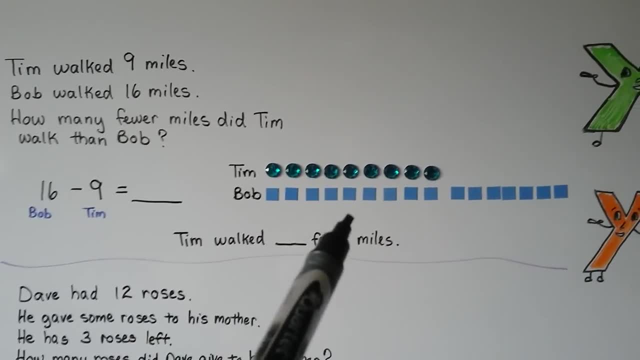 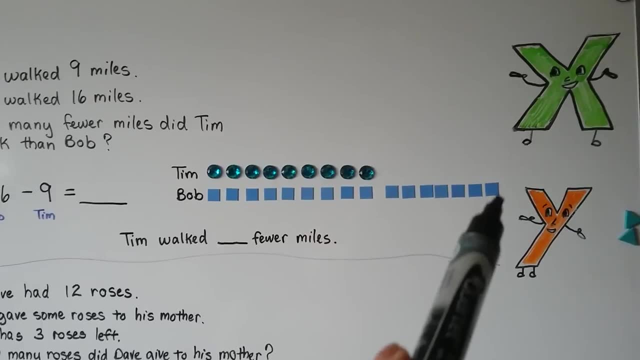 1,, 2,, 3,, 4,, 5,, 6,, 7,, 8,, 9. 10. Even 10.. 11,, 12,, 13,, 14,, 15,, 16.. 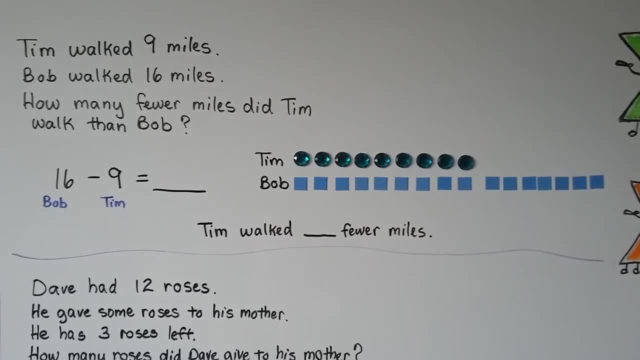 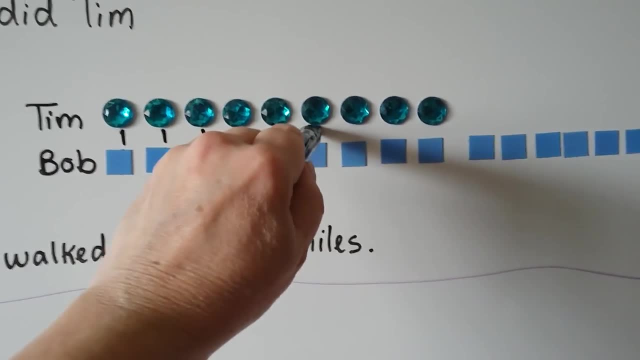 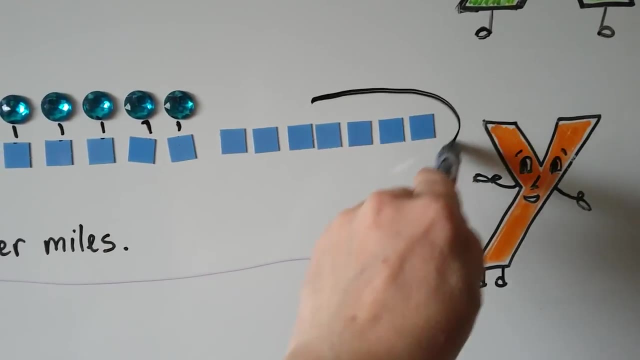 We can compare the counters that Tim has to the ones Bob has And you can see that these all match each other as the same number, And Bob has this many more than Tim, Which means Tim has that many fewer. And how many counters are there? 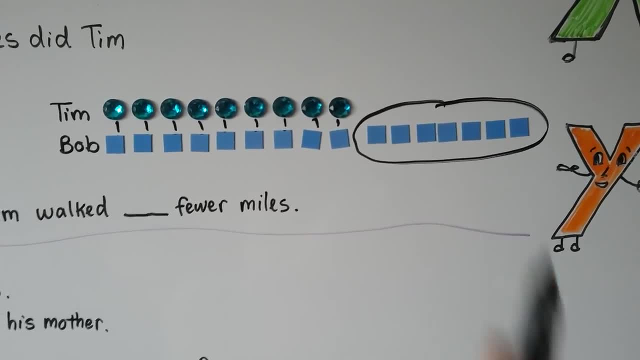 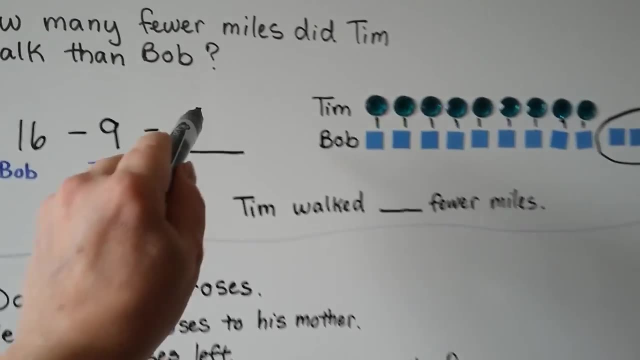 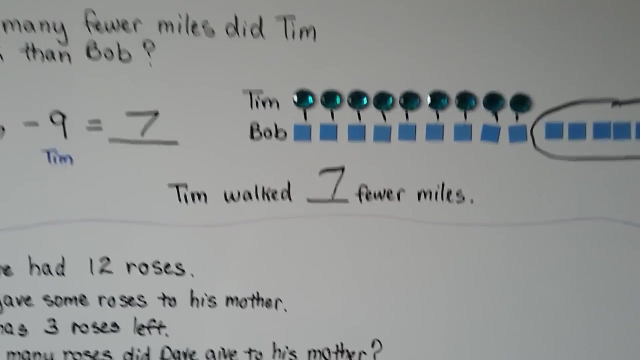 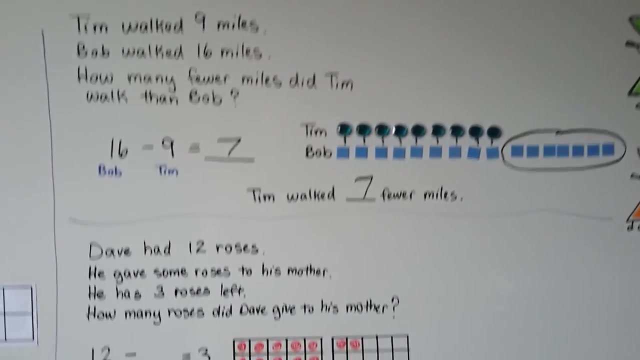 1,, 2,, 3,, 4,, 5,, 6,, 7.. So 16 minus 9 is equal to 7.. Tim walked 7 fewer miles. We just compared the counters next to each other. Dave had 12 roses. 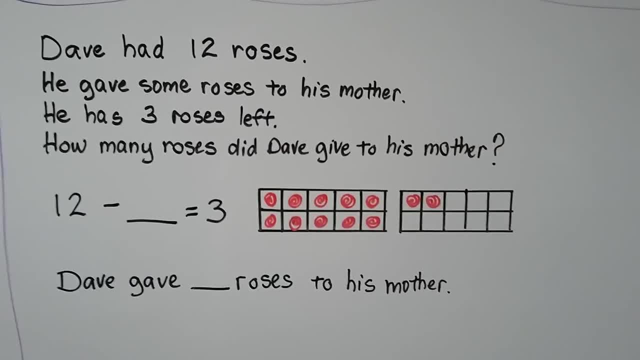 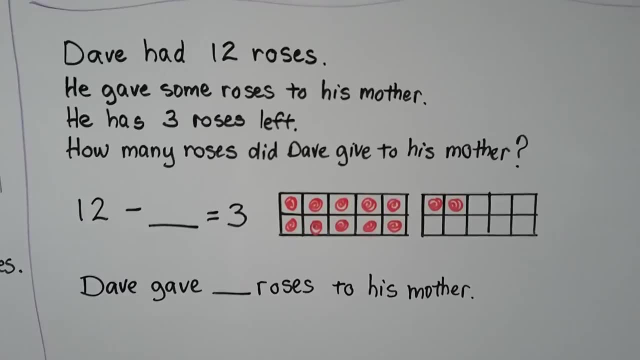 He gave some roses to his mother. He has 3 roses left. How many roses did Dave give to his mother? So what do we need to find? We need to find how many roses Dave gave to his mother. What information do we need to use? 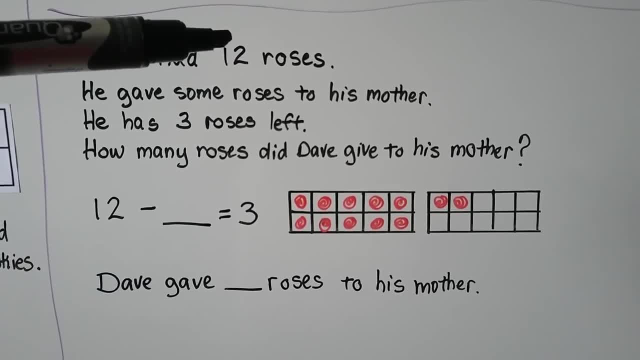 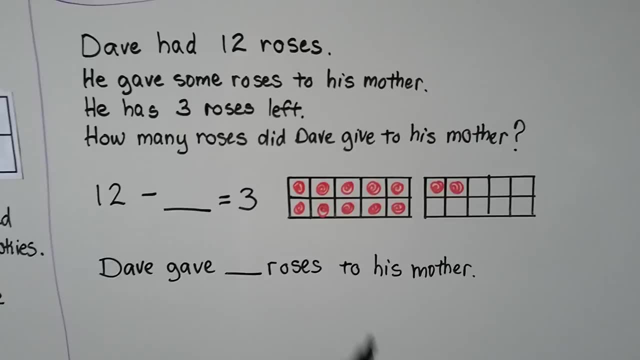 Well, we need to use 12 roses- is how many he had- And he only has 3 left. And how will we use this information? We can use a 10 frame and make counters for roses. Here's 10,, 11,, 12.. 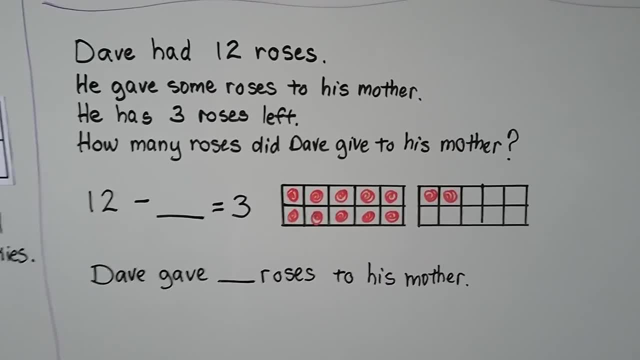 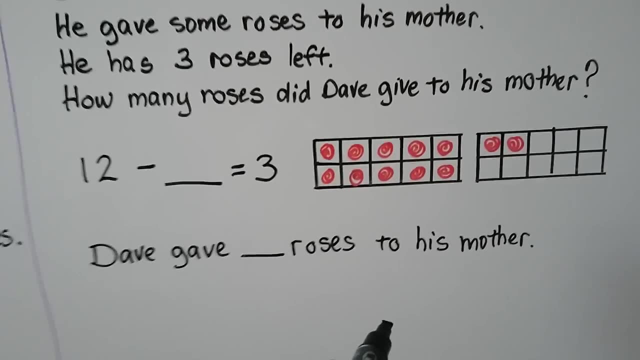 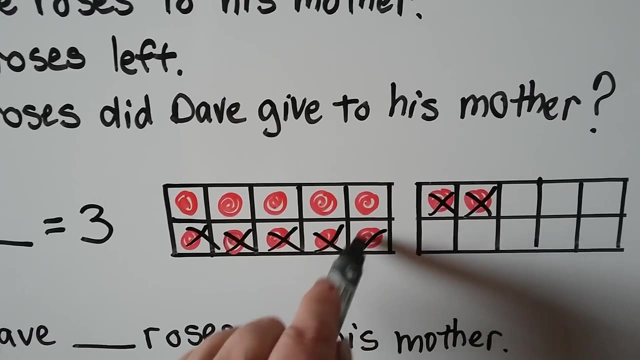 That would be the 12 roses, And if he only has 3 roses left, we can cross out and take away counters. until there's only 3 left, We can take away these and these, And we only want 1,, 2,, 3 left. 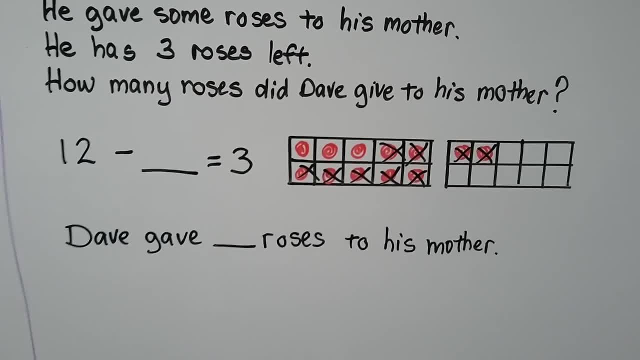 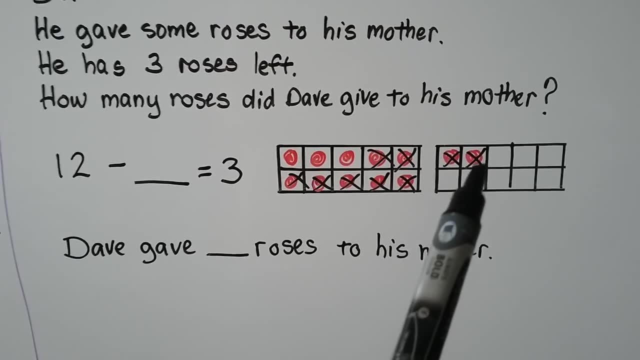 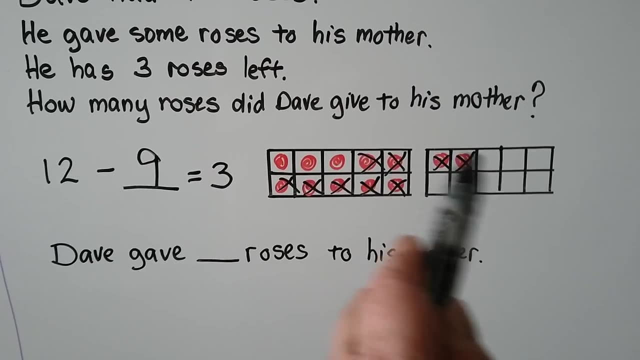 So we still need to cross these out. So how many did we cross out? We crossed out 1,, 2,, 3,, 4,, 5,, 6,, 7,, 8, 9.. That means Dave gave 9 roses to his mother. 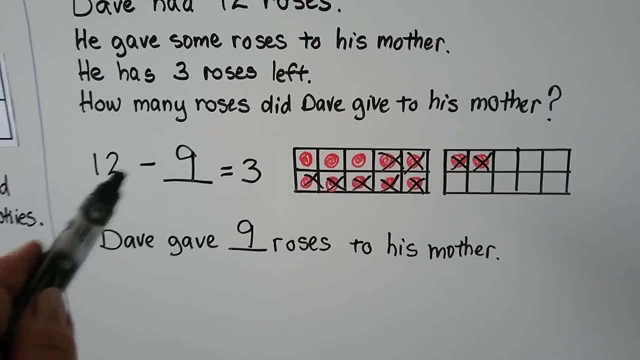 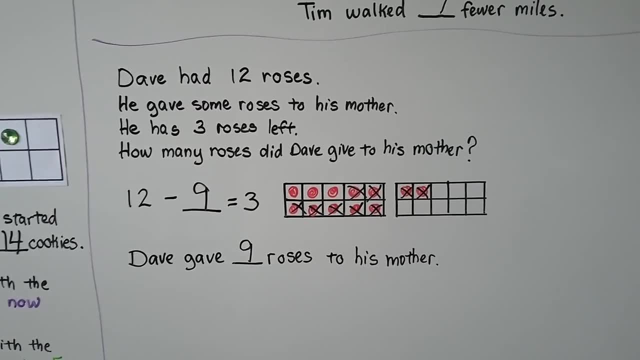 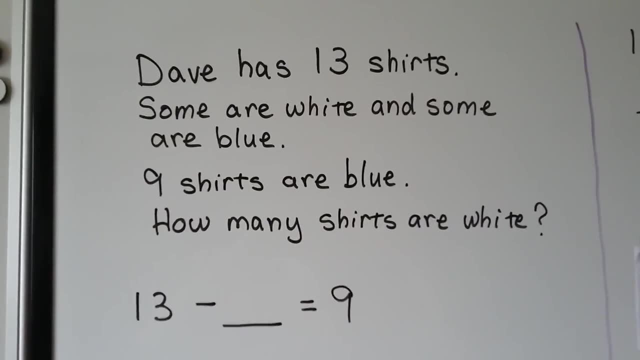 Because he's got 3 left from the 12.. He had 12.. He gave 9 to his mother And now he has 3 left. Now Dave has 13 shirts. Some are white and some are blue. 9 shirts are blue. 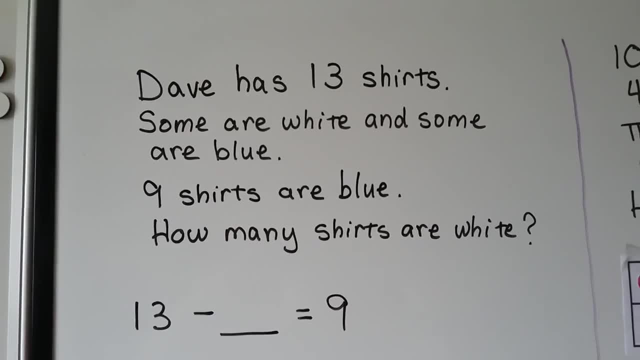 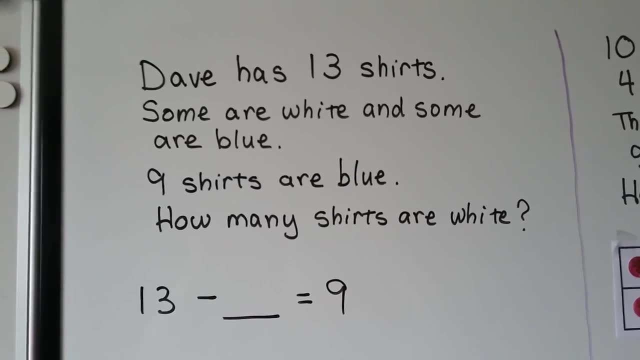 How many shirts are white. So what do we need to find? We need to find how many shirts are white And what information do we need to use. We need to use that. he has 13,, but 9 of them are blue. 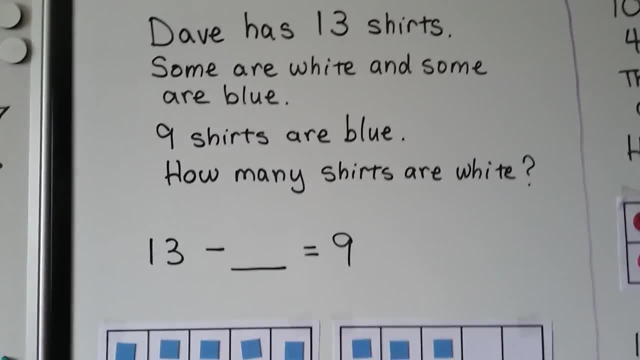 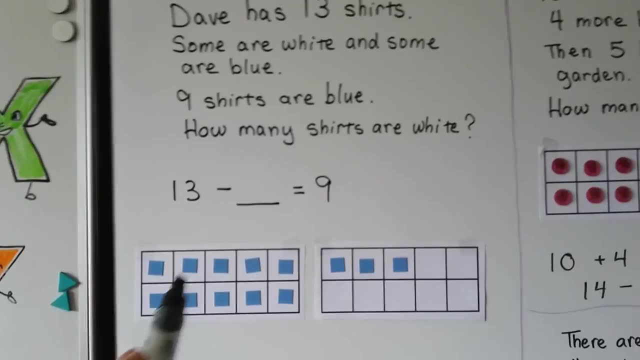 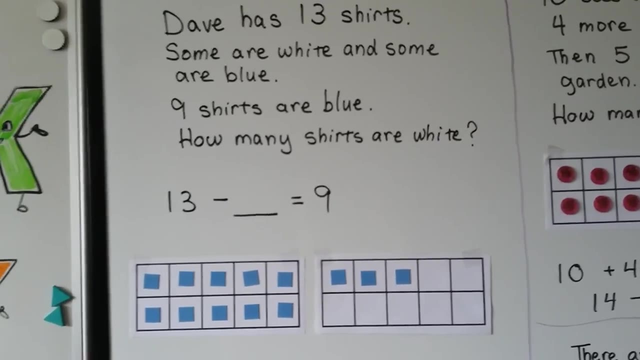 And how will we use this information? Well, we can act it out with counters. We can make 13 counters for 13 shirts: 10,, 11,, 12,, 13.. And we can take away 9 counters for 9 blue shirts. 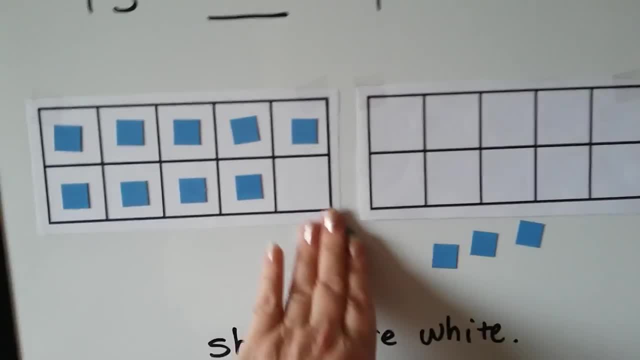 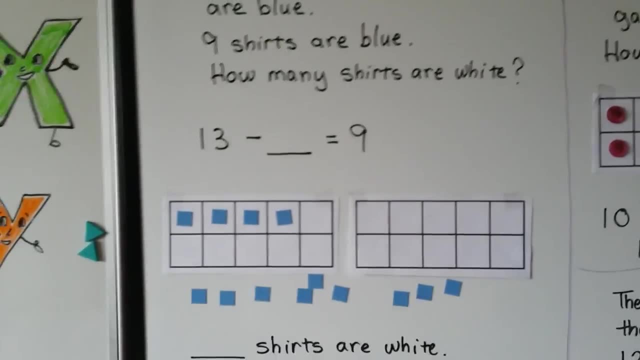 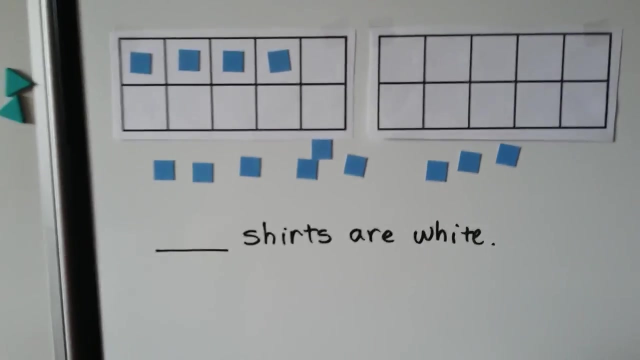 1, 2, 3,, 4,, 5,, 6,, 7,, 8, 9.. How many are left in the 10 frame? 4.. 4 shirts are white. We took away the 9 blue counters for 9 blue shirts. 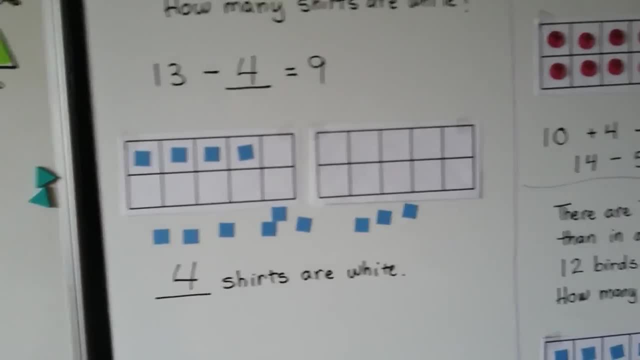 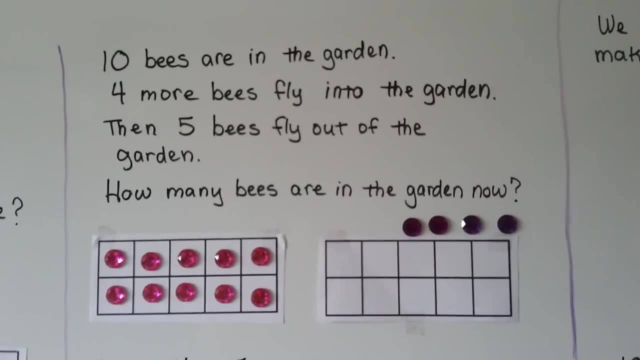 And it left 4.. This one's going to be a little trickier. See if you can do this with me. 10 bees are in the garden, 4 more bees fly into the garden, Then 5 bees fly out of the garden. 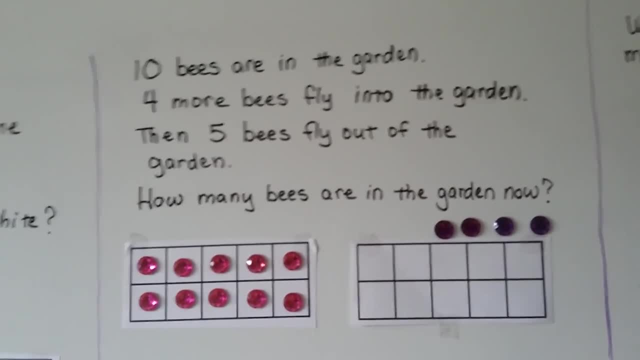 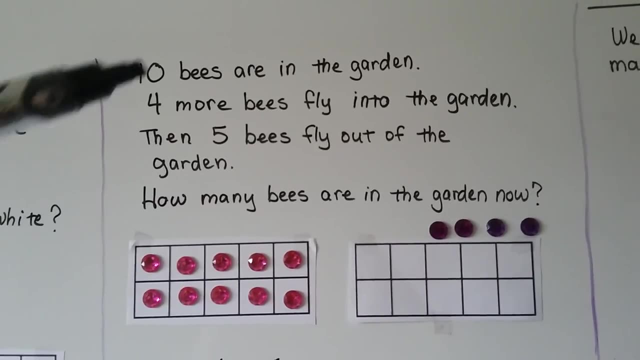 How many bees are in the garden now. So what do we need to find? We need to find how many bees are in the garden right now, And what information are we going to use? We're going to use that. there were 10, then 4 more came and then 5 left. 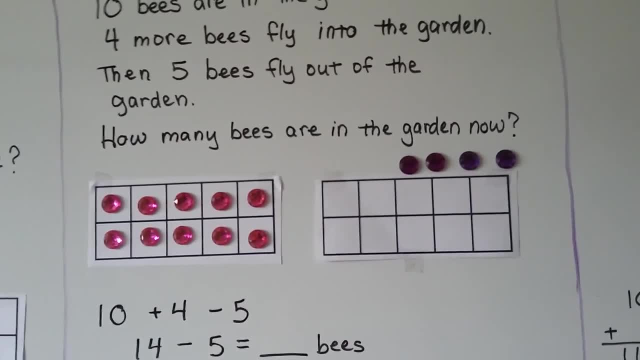 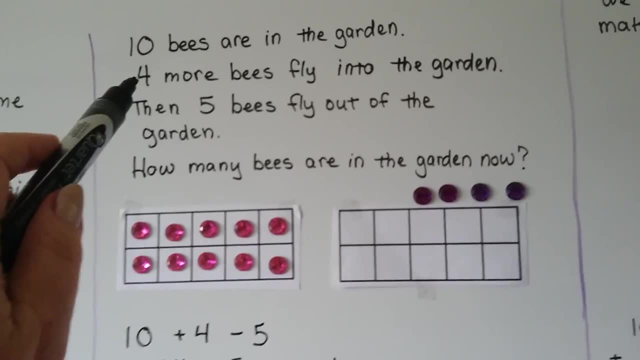 And how will we use this? Well, we can use counters to help us. There were 10 bees, so we have 10 pink gems for the 10 bees in the garden And it says: 4 more bees fly into the garden. 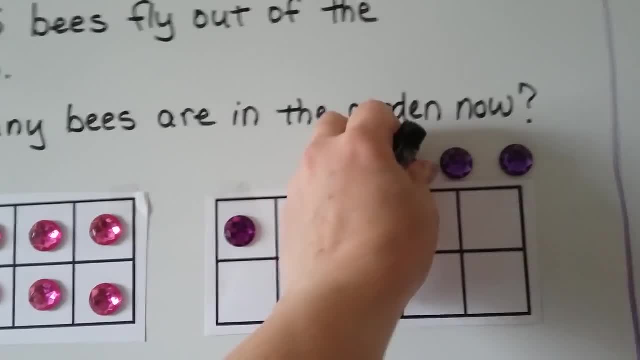 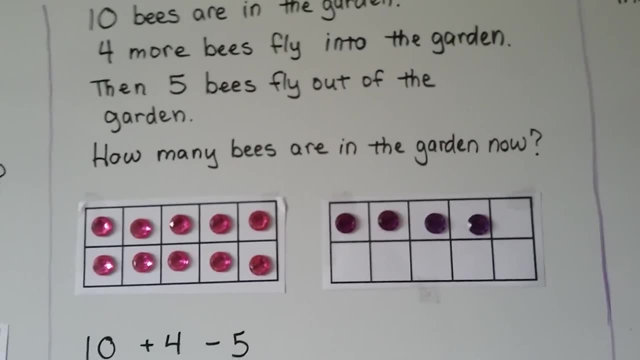 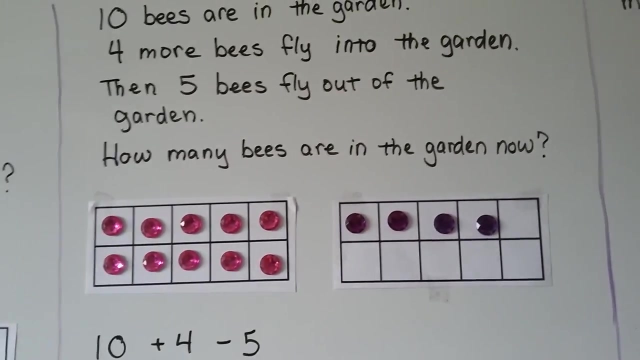 So we can put 4 more counters in another 10 frame: 1,, 2,, 3,, 4.. Now how many bees are there? There's 10,, 11,, 12,, 13,, 14.. Then it says: 5 bees fly out of the garden. 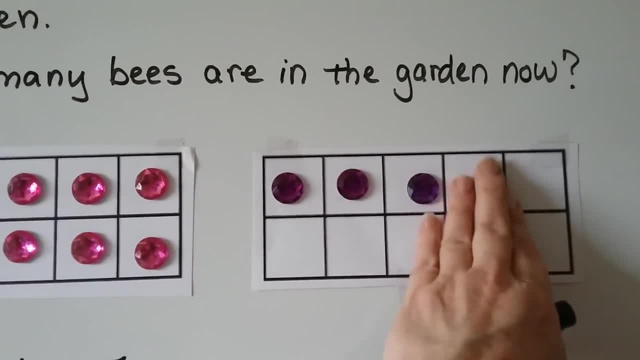 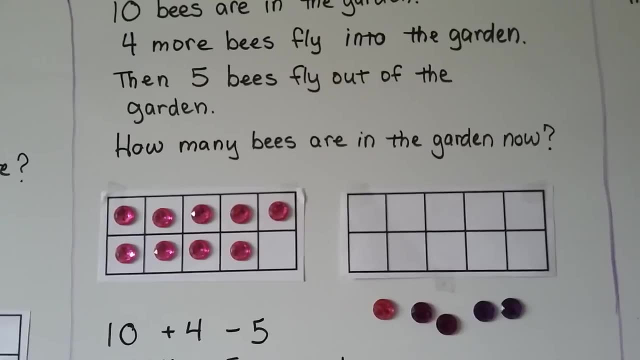 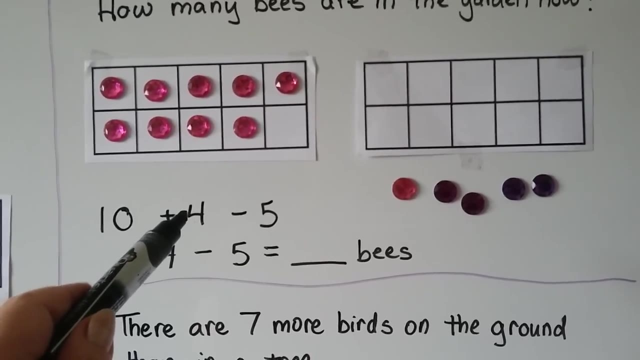 That means we need to take 5 counters away. We take away 1,, 2,, 3,, 4,, 5.. And how many counters are left over 9.. We had 10 bees in the garden. 4 more came into the garden, then 5 left the garden. 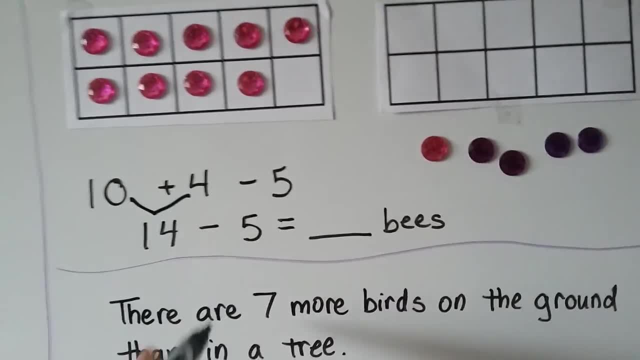 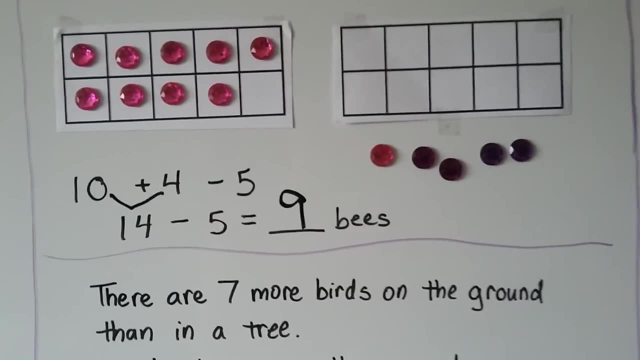 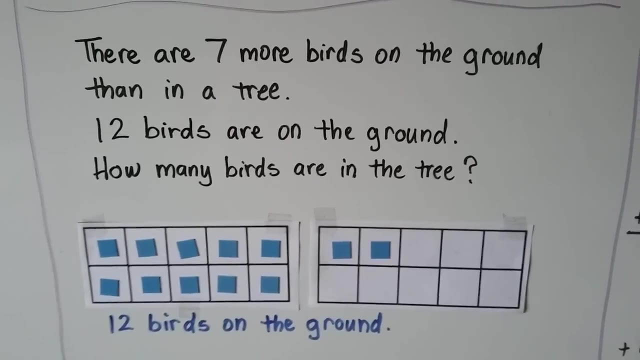 10 plus 4 is 14.. 14 minus 5 is 9.. 9 bees are still in the garden. See if we can do this tricky one. There are 7 more birds on the ground than in the tree. 12 birds are on the ground. 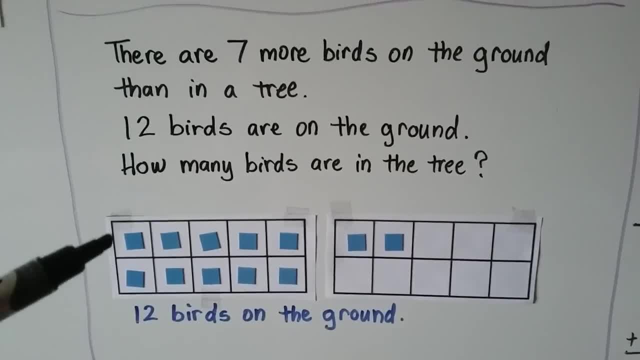 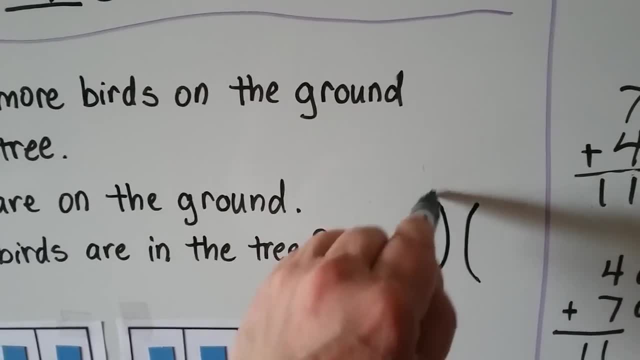 How many birds are in the tree. What do we need to find? We need to find how many birds are in the tree. We can even do a drawing to help us act it out, couldn't we? We could draw a tree And it says there's 12 birds on the ground. 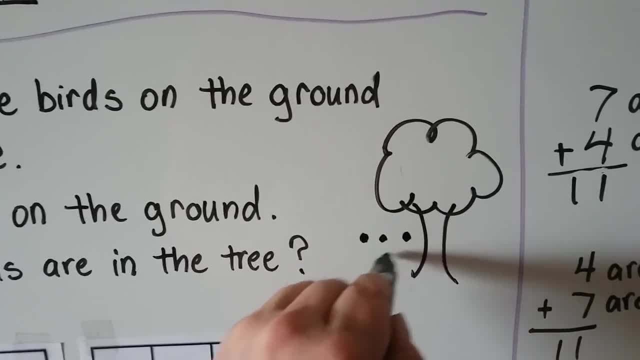 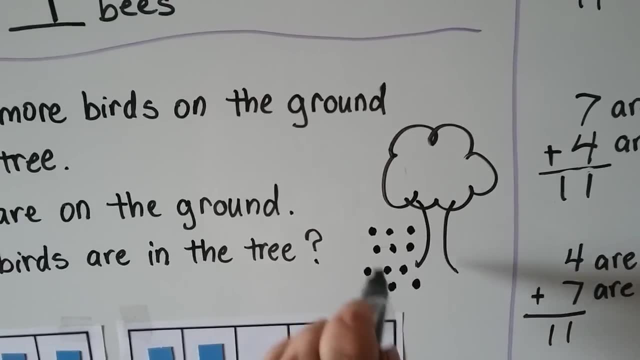 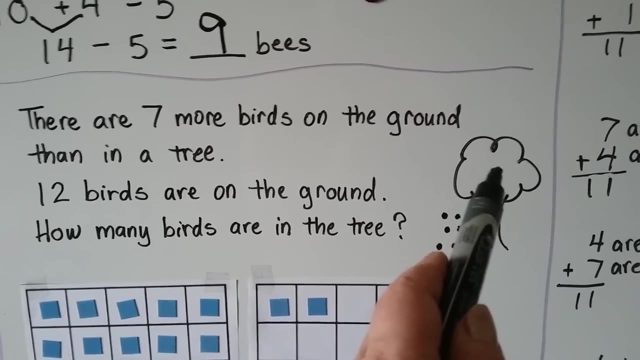 So we could make 12 dots And say that those are the ones on the ground And it says there's 7 more birds on the ground than in the tree. So that means there's less in the tree. We can use counters to help us. 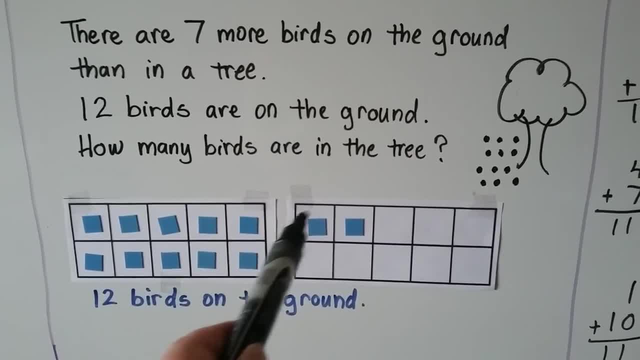 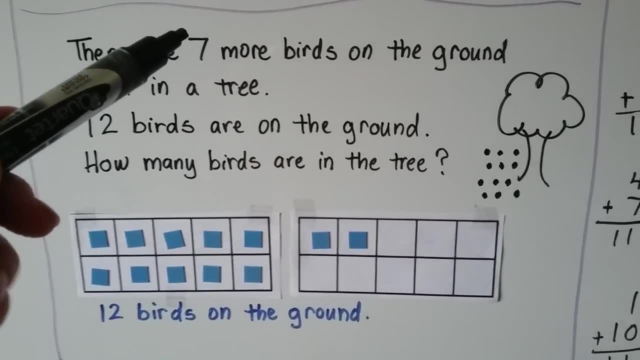 We could say that these 12 counters- 10,, 11,, 12, represent the birds that are on the ground, And if there's 7 more on the ground than in the tree, we could take 7 of these counters away. 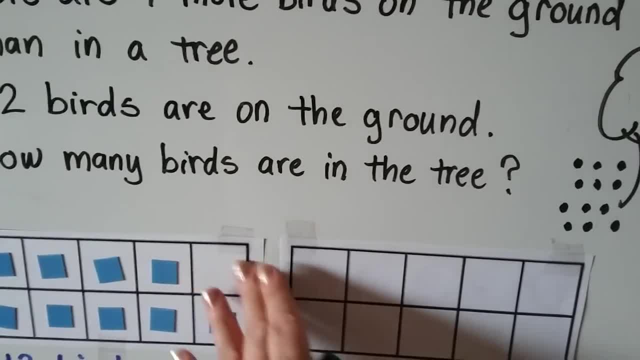 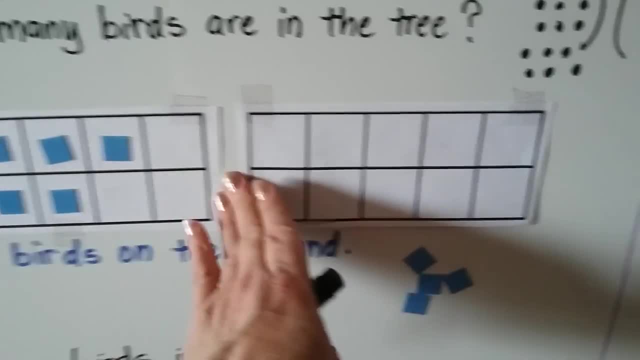 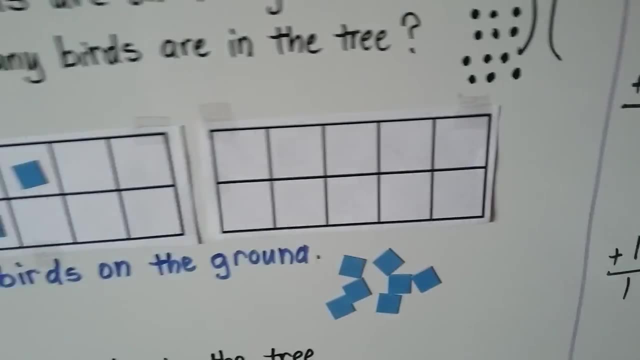 And that will tell us how many are in the tree. Let me move this out of the way, Sorry. And one more. There we go. We took away 1,, 2,, 3,, 4,, 5,, 6, 7 counters. 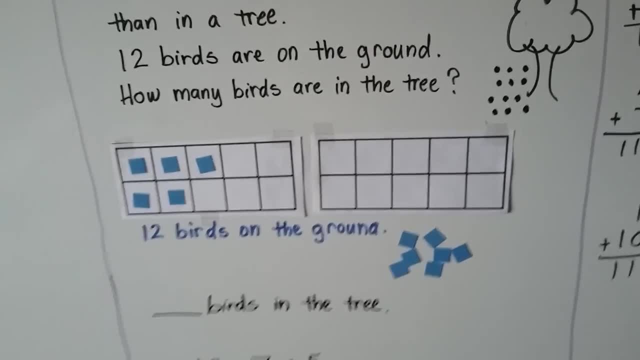 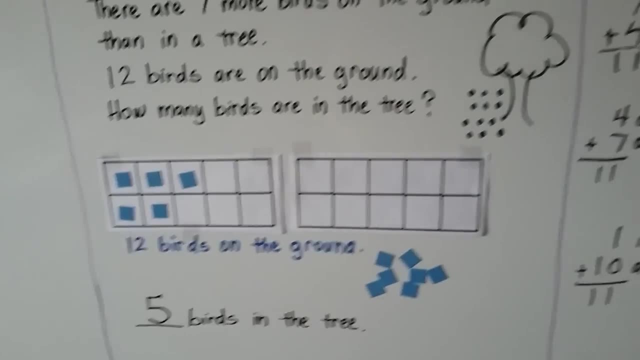 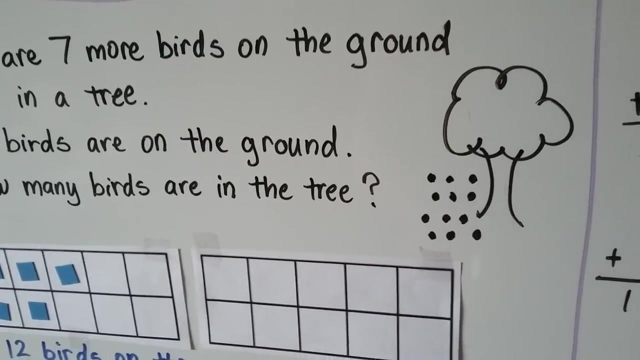 That left us with 5.. That means there's 5 birds in the tree. 12 minus 7 is equal to 5.. If this is our tree and these are the birds that are on the ground, and there's 7 more on the ground than in the tree, 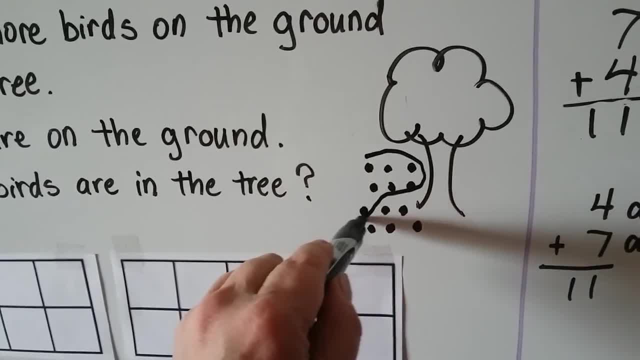 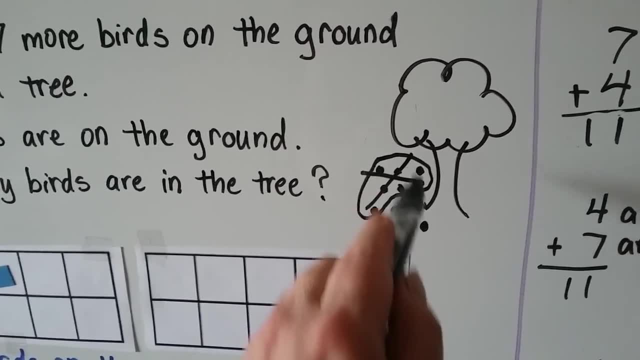 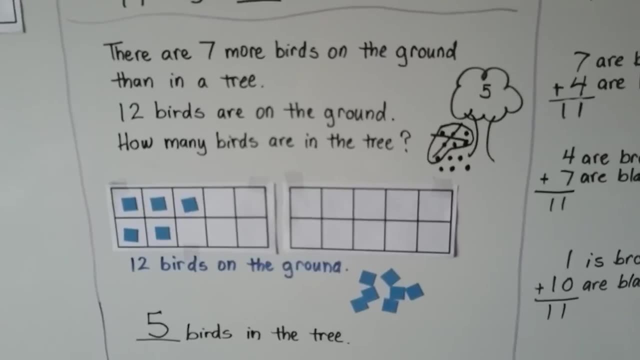 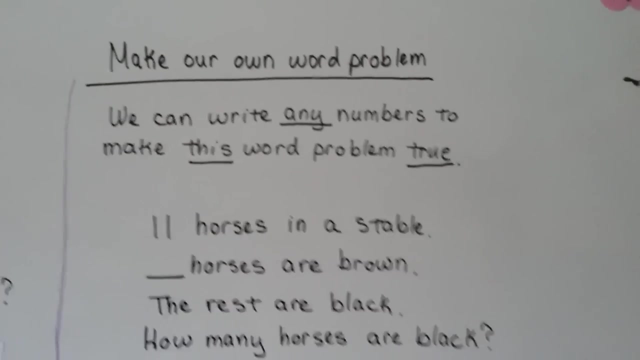 we can take away 7 of them And we have 1,, 2,, 3,, 4, 5 left over. That means there's 5 in the tree. We can make our own word problem. We can write any numbers to make this word problem true.